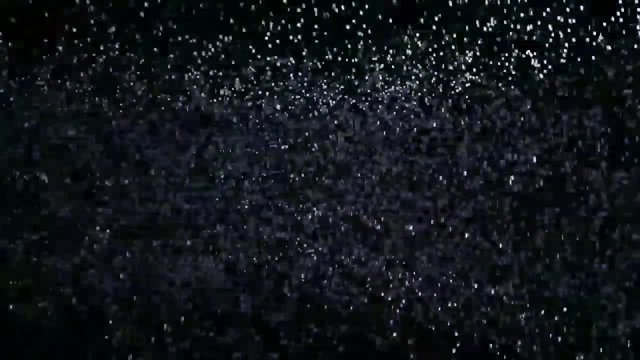 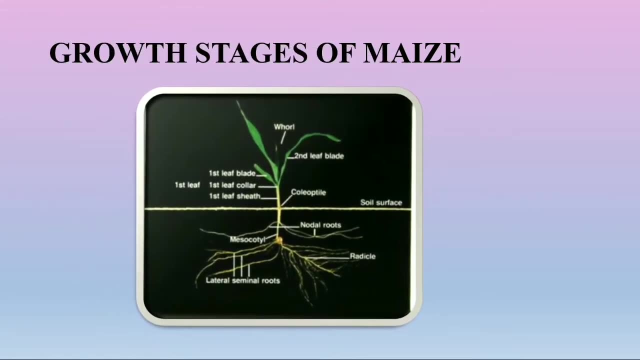 Before going to the growth stages of maize, let us discuss some of the parts which are included in the maize. Let us see the roots- roots like lateral seminal roots, radical nodal roots, and we have the mesocotyle, after that colioptile, which arises from the soil and bearing the first leaf shade. 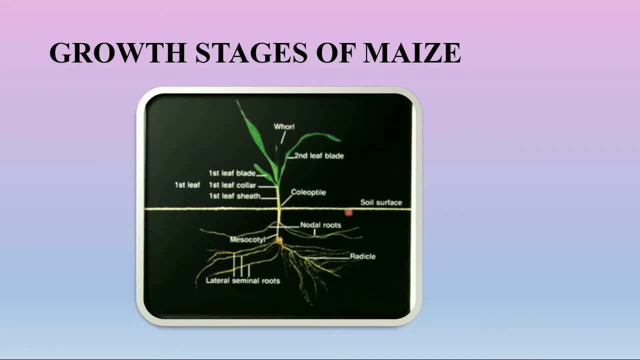 You can observe here in the image, It is showing the first leaf sheath, first leaf collar and first leaf blade. Here you can clearly observe what are the sheath, collar and blade And this is the soil surface Before going to the growth stages of maize. some people are asking about the PDF. 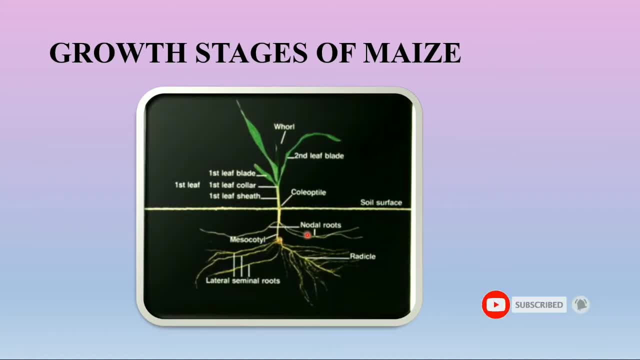 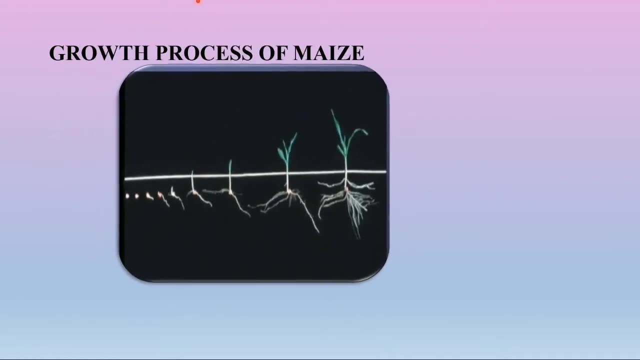 I will give this PDF in the description box and you can observe it and study carefully And grow the knowledge of the maize crop. In the growth process of the maize we can see the seed, how it is emerging and colioptile. 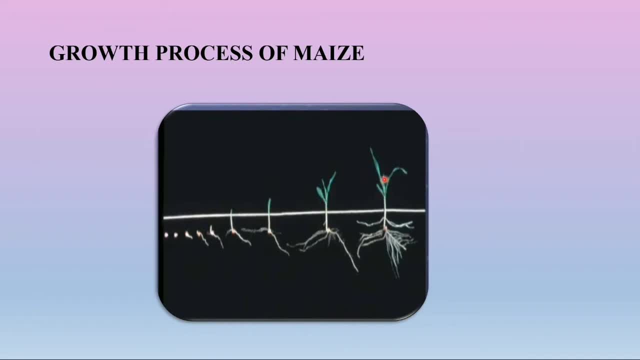 And you can see the collar and the leaves above the soil surface and the plant is growing. The vegetative stages, or some of the stages, which are described using the leaf collar method, Which is defined by the number of collars on the plant Leaves, are counted from the lower most part and to the upper most leaf with the leaf collar. 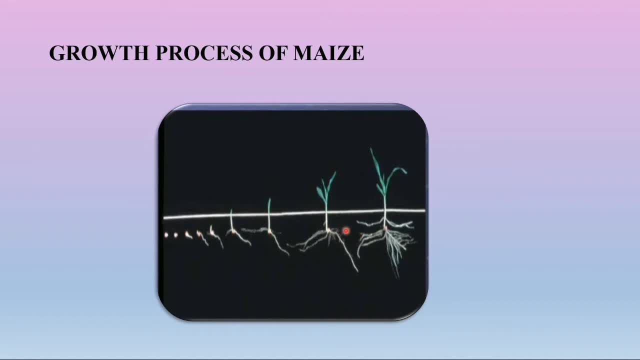 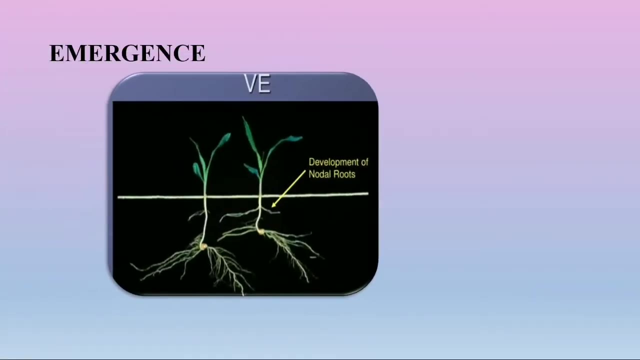 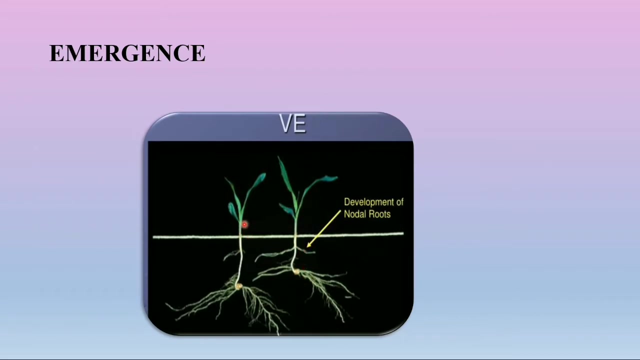 Which is the connection between the leaf blade and the leaf sheath, The leaves in the hole that are not fully expanded or not counted. Let us discuss about the emergence Here. you can observe in the image the emergence of the plant, The colioptile leaf, the first leaf visible. 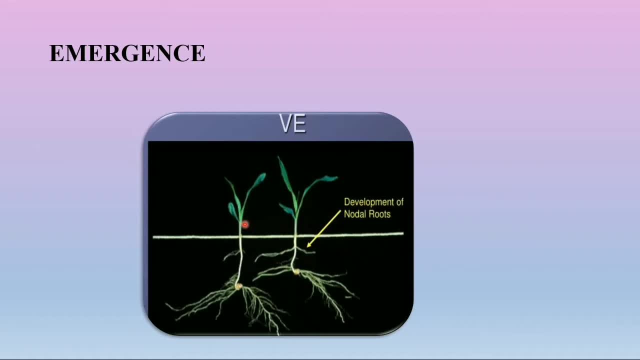 This leaf will be shorter than the lateral emerging leaves and has the rounded tip. The growing tip of the plant should be 1 to 1.75 inches below the soil surface And the seminal roots begin growing from the seed, The permanent nodal roots. here you can observe the nodal system will begin developing at this point. 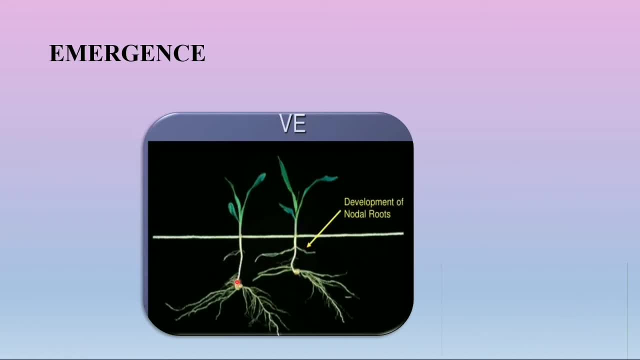 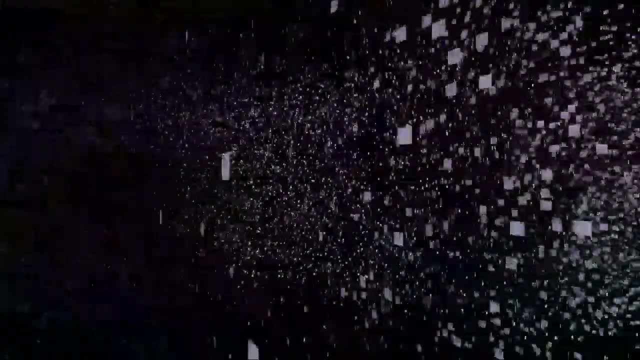 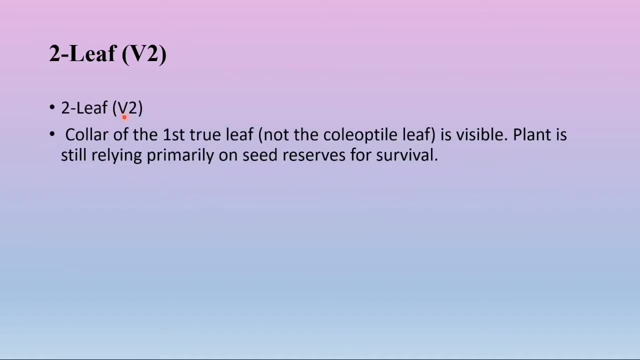 If the seed is planted too shallow, The root system will have a difficult time becoming established. The second leaf stage. Let us discuss about what is the second leaf stage. The collar of the first true leaf, not the colioptile leaf, is visible in this stage. 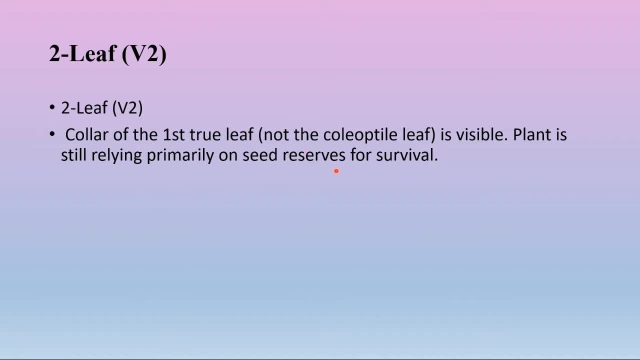 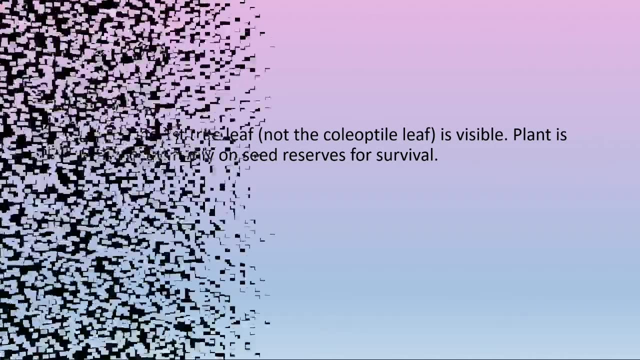 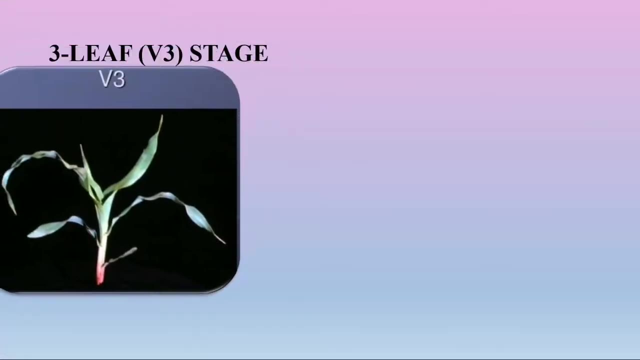 And the plant is still laying primarily on the seed reserves for the survival. This is the second leaf stage of the seed, The grays of the maize. Next coming to the third leaf stage. Here we will be seeing the three leaves. It is showing that the growing plant 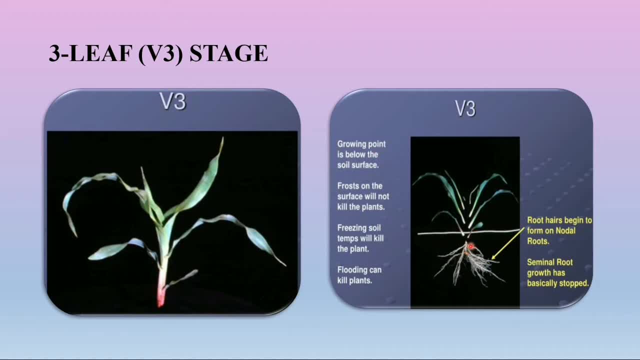 Growing point below the soil surface. Frost on the surface will not kill the plants. Freezing soil temperature will kill the plants. Flooding can kill the plants, So care should be taken. flooding should not occur in this crop and root heads begin to form on nodal roots and seminal 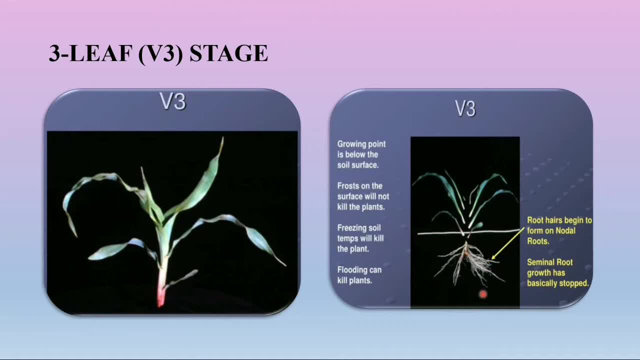 roots. growth has basically stopped here. you can see that on the nodal roots we are seeing the root heads in this third leaf stage of the maize crop and the color of the third leaf is visible. occurs appropriately at 10 to 14 days after the emergence and growing point below the soil. 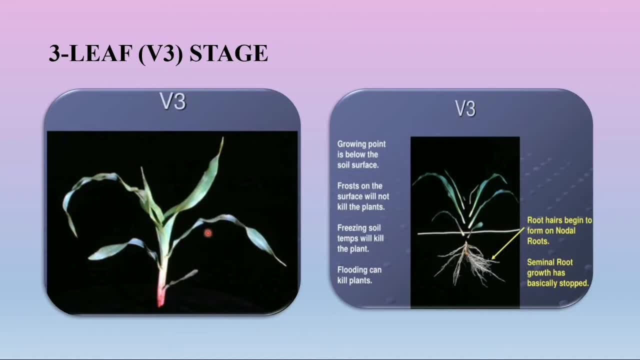 surface the plants, total leaf number and ear shoots are developing. in the stock. the photosynthesis is now very active and supporting the plants having the leaves and may apply to 4d or dicamba from emergence through the fifth leaf stage without the drop nozzles, and coming to the next stage. 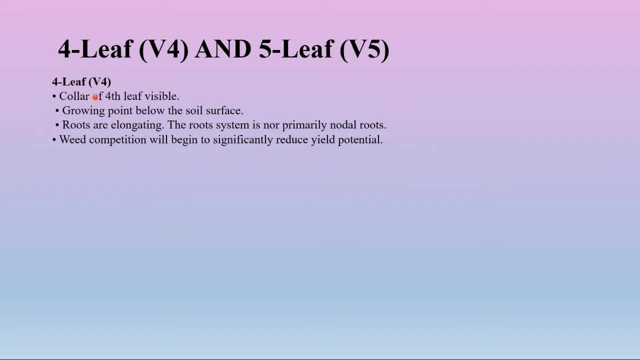 fourth leaf and fifth leaf stage. we have the fourth leaf stage. we can observe the color of the fourth leaf visible and the growing point below the soil surface. roots are elongating. the root system is not primarily nodal roots. weed competition will begin to significantly reduce the 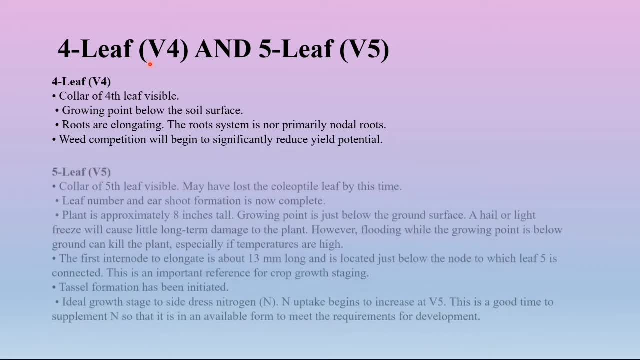 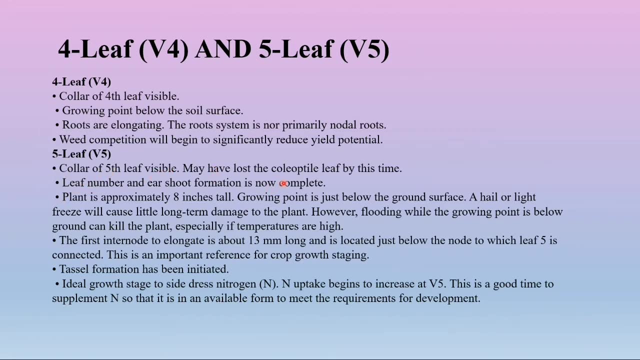 soil potential. in the fourth leaf stage of the maize and fifth leaf stage of the maize we can observe the color of the fifth leaf and it may have lost the colioptile leaf by this time. at the fifth leaf stage, the leaf number and the ear shoot formation will be completed in. 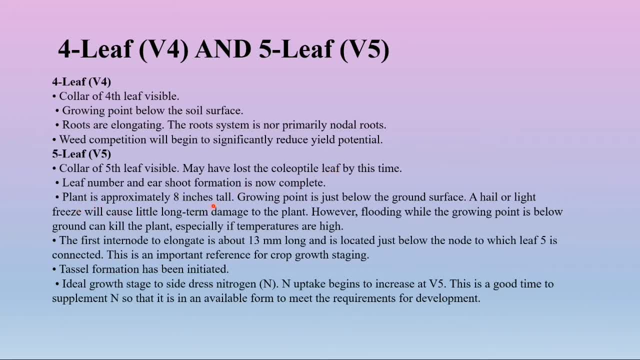 this stage and the plant is approximately about 8 inches tall. in fifth leaf stage the growing point is just below the ground surface and the hair or light freeze will cause little long term long term damage to the plant. however, the flooding while the growing point is ground can kill the plant. so flooding should not happen in the crop, so it can kill the plant. 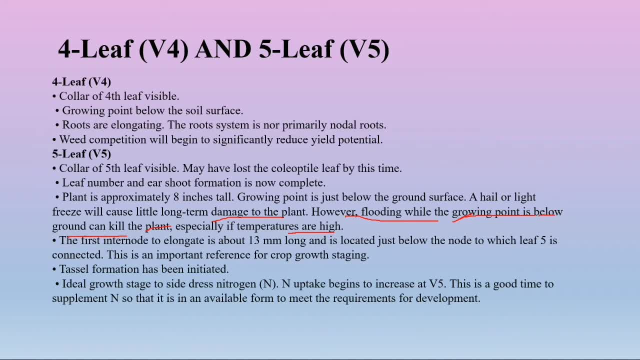 especially if the temperatures are high. the first internode to elongate is about 13 mm long and is located just below the node to which the leaf 5 is connected. this is most important reference for the crop growth. staging and tassel formation has been initiated in the 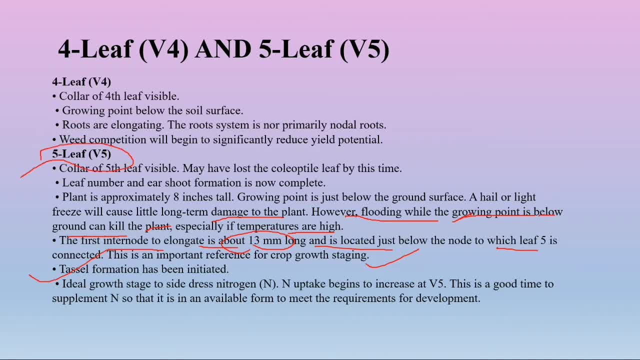 fifth leaf stage you should observe- and ideal growth. ideal growth stage to side dress nitrogen: nitrogen uptake begins to increase at v5. that is fifth leaf stage. this is a good time for the supplement of the dose of nitrogen so that it is an available form to meet the requirements for the 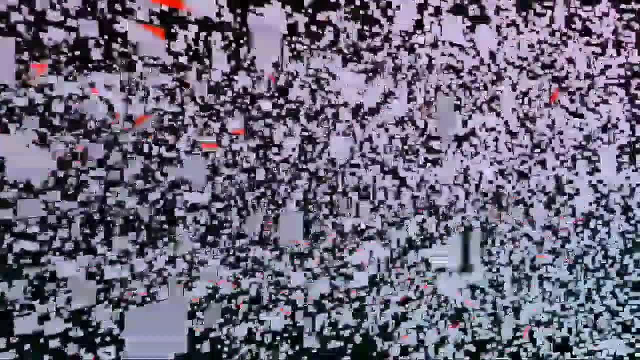 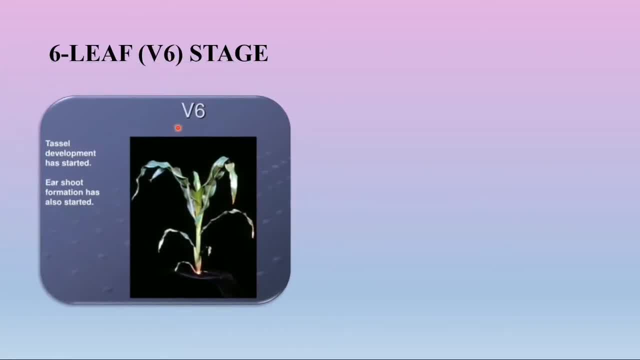 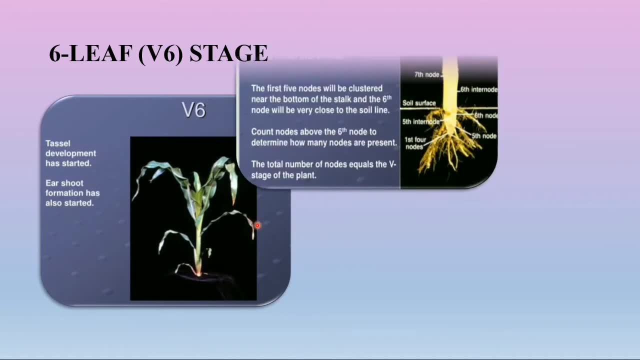 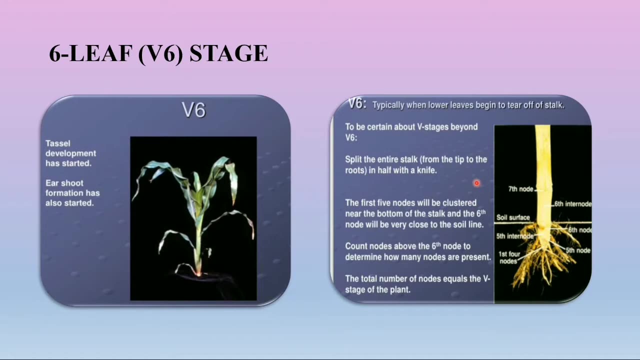 development of the crop growth stage. here in the sixth leaf stage, you can observe the collar of the sixth leaf and occurs approximately three weeks after the emergence. the growing point will be growing point and the tassel above the soil surface making the plant move, venerable to hail or freeze the permanent root. 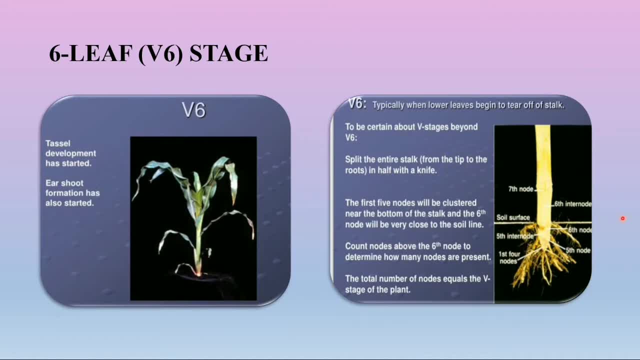 system, rather than this mannose, is now the primary root system supporting the plant, and the root system extends approximately 18 inches in the 6th leaf stage, and here you can observe the tillers are may developing at this stage and internode elongation also occurs in this sixth leaf stage. 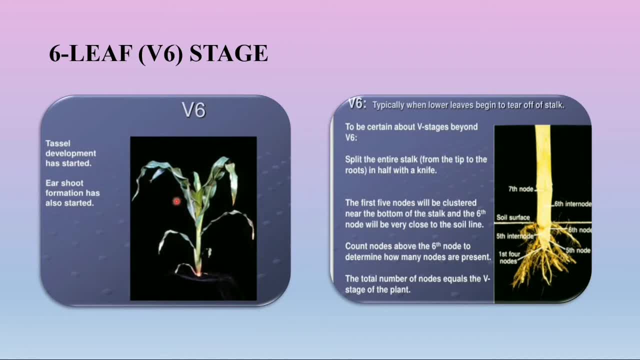 and the continue to check the roots for western corn root form larvae. continue to check for small, Don't touch many fat trees if left at home colony so that you have enough time to grow to see the Saya tree. This root tree may wait for 12 months to die. 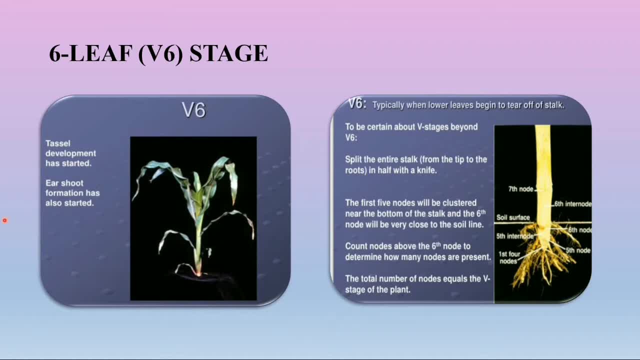 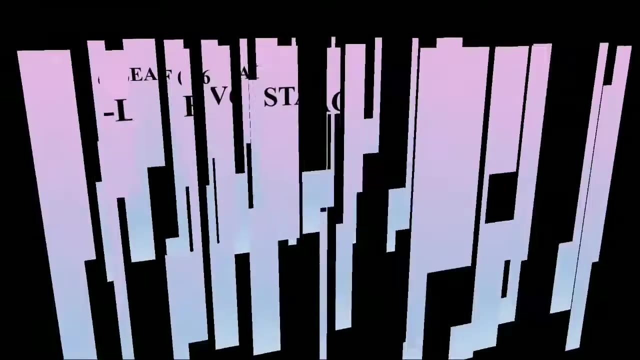 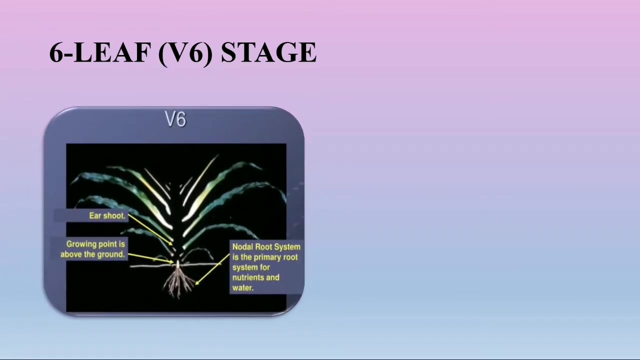 of banks, grass mites. it may affect the crop at this stage. so this stage you should be careful and observe all this: mites and larvae is occurring or not. as we discussed earlier about the sixth leaf stage, you can see here in the image we are having. 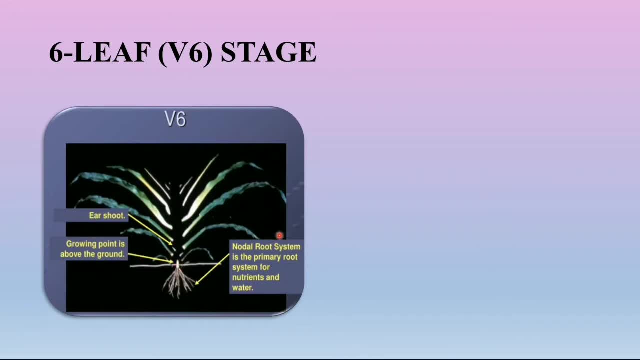 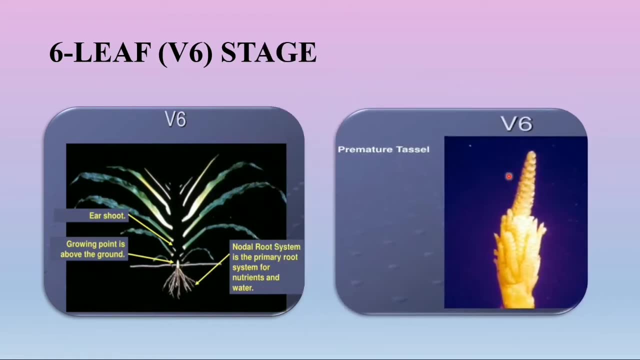 the ear root growing point is above the ground level and the nodal system will be playing a primary root system for the nutrients and the water and also the development of the premature tassel, also observed in the sixth stage, as you can observe here in the image, like this: 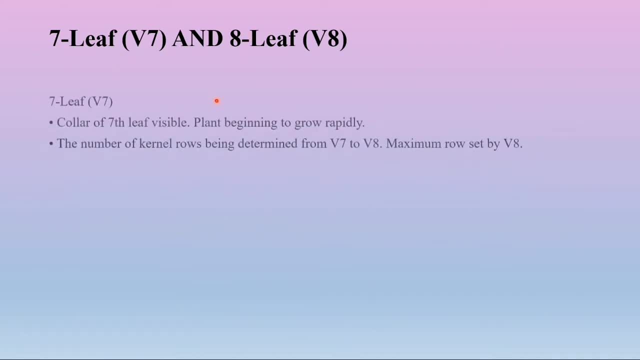 after the sixth leaf stage. you can observe the seventh leaf stage and the eighth leaf stage where we are having the seventh leaf stage. we can observe the color of the seventh leaf. seventh leaf and the plant beginning to the grow rapidly and fast, the number of kernels also. 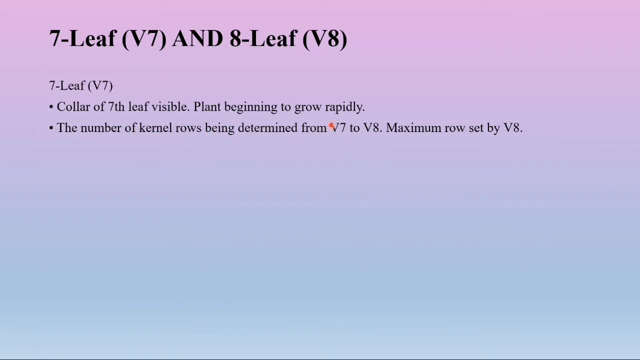 grow, kernel rows being determined from the v7 to the v8 maximum row set by the eighth leaf stage and in eighth leaf stage you can observe the color of the eighth leaf and it approximately of 45 days after the emergence may have lost lower two leaves. 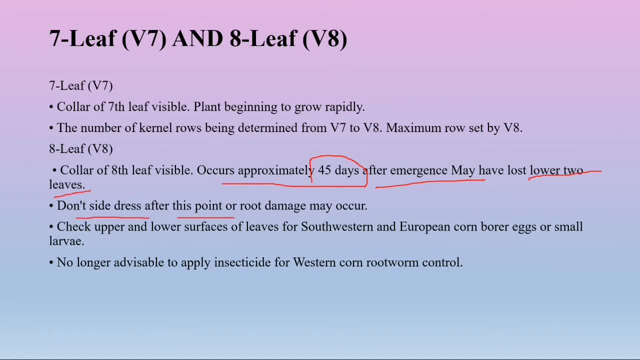 don't do not side dress after this point or root damage may occur. check upper and lower surfaces of the leaf for western, southwestern and european corn borers x or small larvas no longer advisable to apply. insect sites for western corn rootworm control. in the ninth leaf stage you can observe the color of. 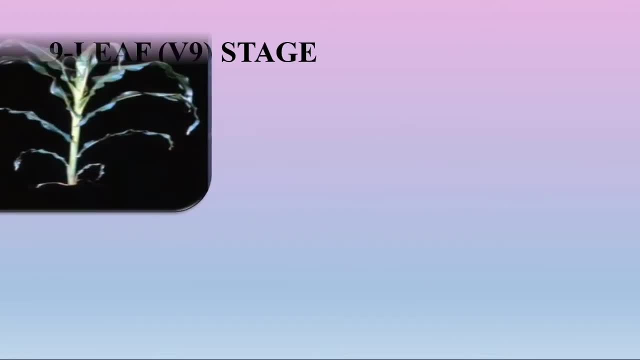 rejected piece file and another ear shoots for non proprietors. another shift in the development and you can observe here that the worship for of the ninth leaf and also the song shoot is seen in the leaf calldend one of the external movement through the central vocal cords, seen in the leaf called pre. a canal tool is also visible here in the this sign Father von Orel � call by stop and this call can be 지금 komplett imbeliert carry around the of the leaf which is turning comes into operation in conflict with our balance of light and also plant policies and contactsea efficient band of the types of water flow so 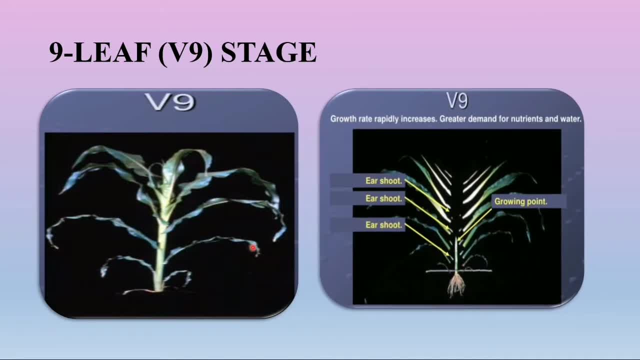 These regions may have up to 8 year shoots. The tassel is rapidly developing and corn borer feeding damage should be evident on leaves in the whole of the infested plants. Here we can observe in the 9th leaf stage. the growth rate rapidly increases in this stage and the greater the demand for the nutrients and the water in this stage, mainly as it is the growing point of the crop. 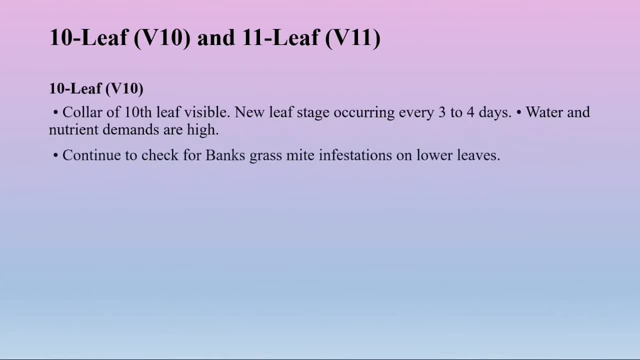 Here you can observe the 10th leaf and the 11th leaf stage. In the 10th leaf stage the color is visible of the 10th leaf and new leaf stage occurring every 3 to 4 days. Water and nutrients are visible in the 10th leaf stage. 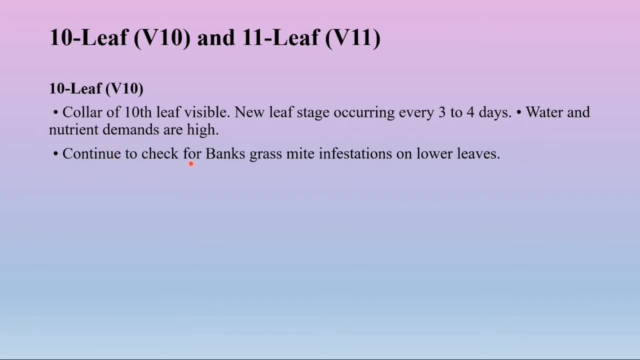 nutrient requirements are high. continue to check for the bank grass mites infestations on the lower leaves in the 11th leaf stage. the color of the 11th leaf is visible and may have lost the three last. the lower three leaves and a few corn borers will have entered the stock by this time. no longer the feasible. 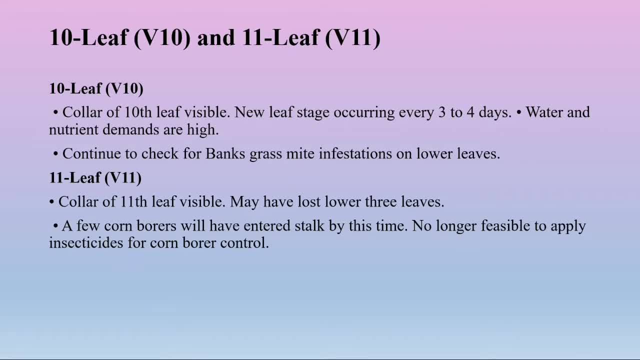 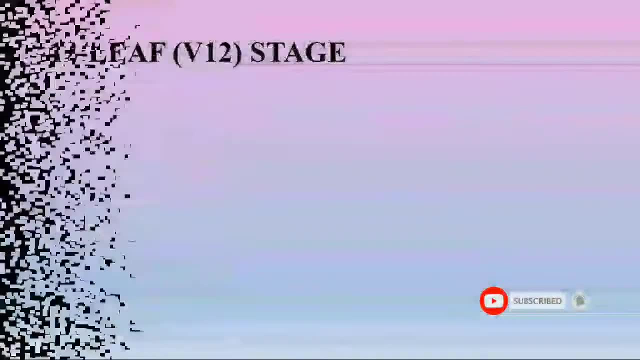 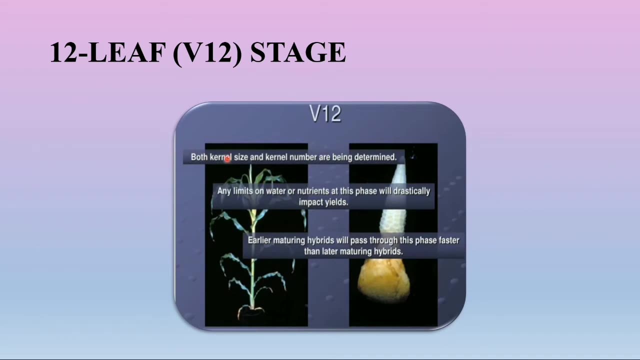 to apply insecticides for the corn borer. coming to the next stage, that is, lead, this 12th leaf stage, you can observe here, in the 12th leaf stage, we are having the both canal size and the canal number are being determined, any limits on water. 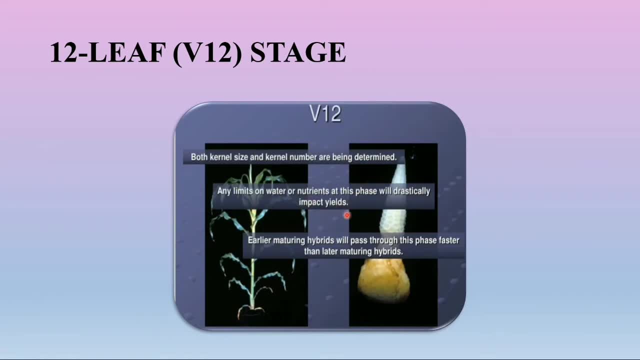 or nutrients at this phase will drastically impact the yield, as in this stage the water and nutrients are most important. if the water and nutrients are less, there maybe increase, there may be reduce in the yields. so the case should be taken into consideration in the following exchange stage for the growing. 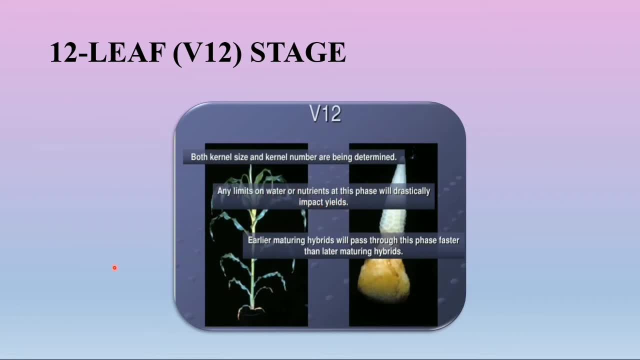 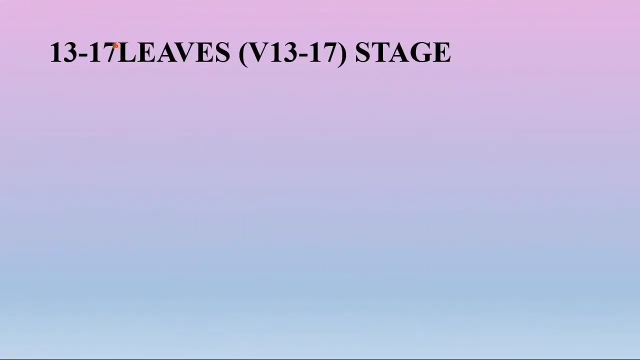 to give water or nutrients at this stage. the earlier maturity hybrids will pass through this phase faster than later maturing hybrids and number of kernel rows already determined. the top year is still smaller than the lower year. shoots coming to the 13-17 stage. V13, V, 17 stage. leaf stages at 13 to 17. 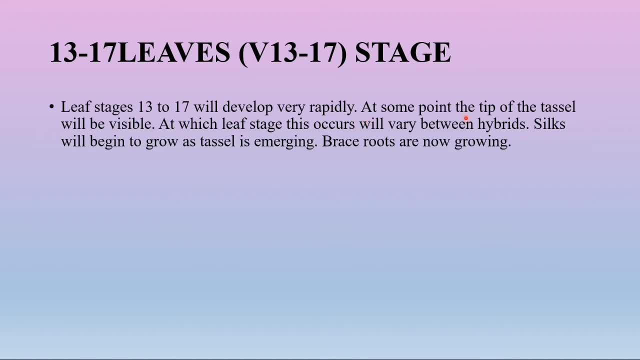 will develop very rapidly. at some point the tip of the tassel will be visible and the leaf stage occurs. very vary between the hybrids and silks will begin to grow as the tassel is emerging. this is the most important point to note that silks will begin to grow as the tassels are emerging. as 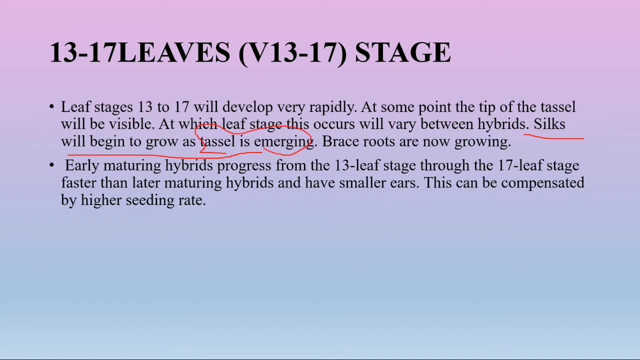 already. tassels are emerging. the silks also will be growing, begin to grow. the early maturity hybrids progress from 13th leaf stage through the 17th leaf stage the faster than the later maturing hybrids and have smaller ears. this is. this can be compensated. 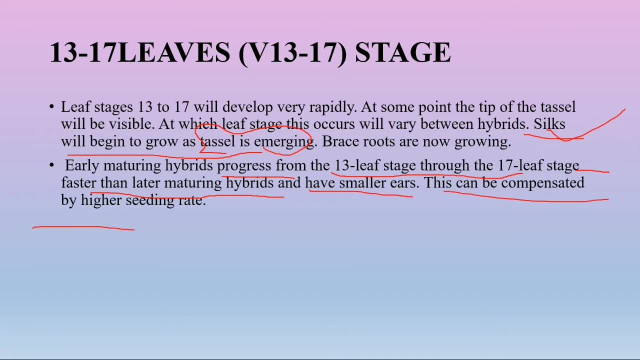 this can be compensated by higher seed rate. next, the attempt should be made to have the soil profile full of water prior to tassel emergence. the care should be taken that the water profile should be with the full of water before the tassel emergence as the braised roots developing. 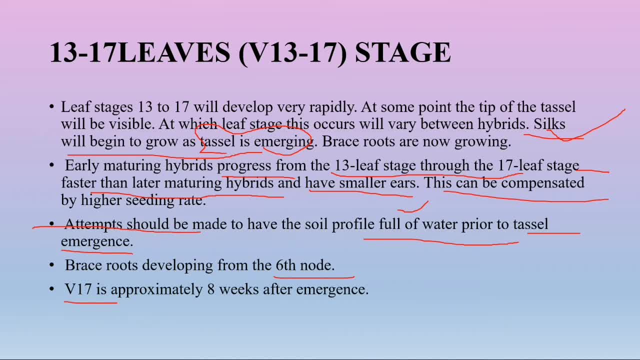 from the silks will begin to grow as the silks will begin to grow, as the silks will begin to grow. the sixth node and v17 is approximately about eight weeks after the emergence. you can observe the v15 at eight weeks after the emergence. the most important. 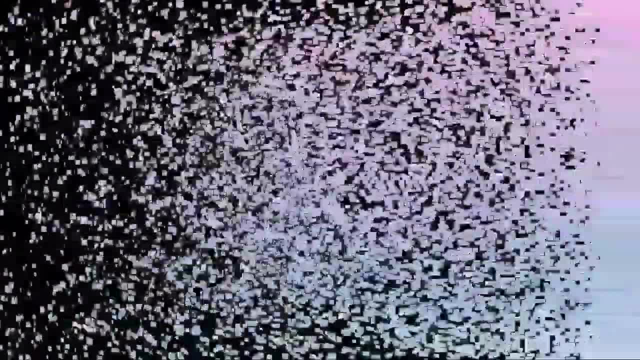 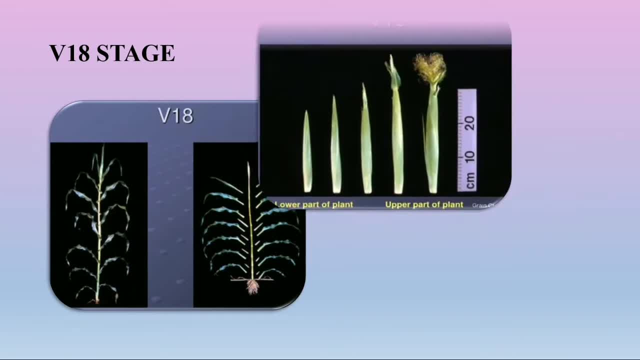 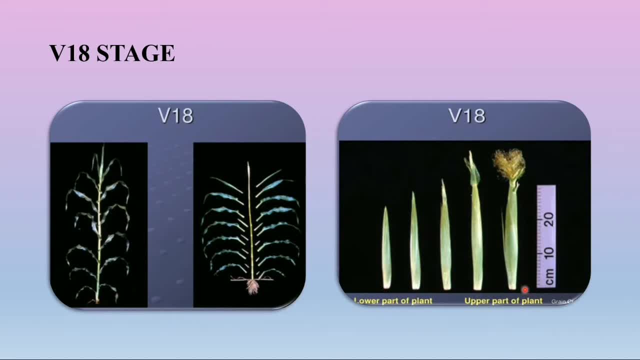 growing and how it is growing and how it is growing and how the difference between the lower part and the lower part and the upper part- upper part of the plant will be the lower part and the upper part- upper part of the plant will be the lower part and the upper part- upper part of the plant will be having the silk like this at this stage. 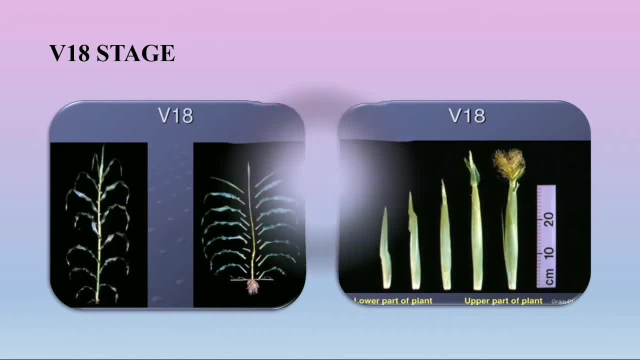 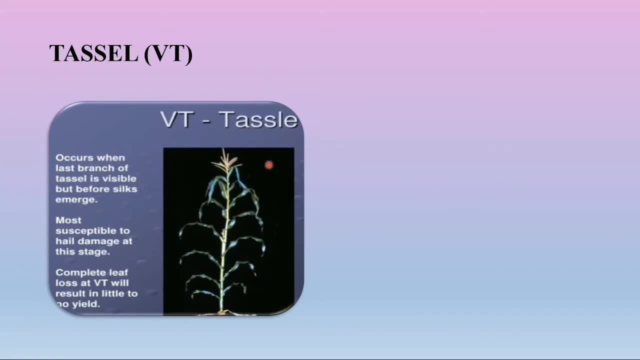 having the silk like this at this stage. having the silk like this at this stage of v18, of v18, of v18 coming to the next stage. tassel stitch vt. coming to the next stage. tassel stitch vt. coming to the next stage. tassel stitch vt, where it shows the tassel is fully emerged. 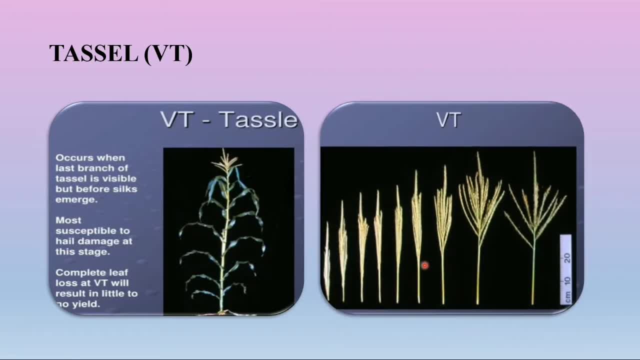 where it shows the tassel is fully emerged. where it shows the tassel is fully emerged at two to three days. at two to three days. at two to three days prior to the silking, the plant is at full height and all leaves have emerged like this in the image, and hail damage is most significant. 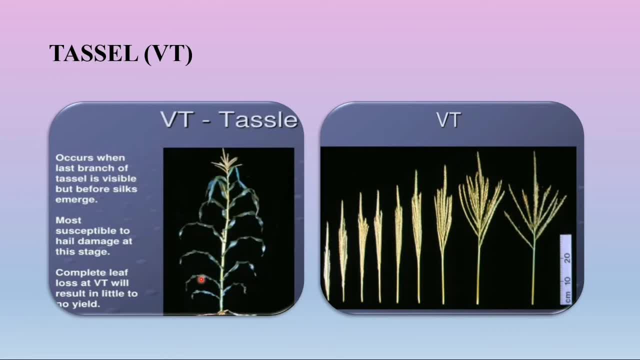 at tasseling and can result in 100 percent yield loss if the tassel is lost, so care should be taken that it should not. the hail should not damage the tasseling stage and beginning of the fourth week period. that is very critical. silking will generally begin in two to three days, stress occurring a few. 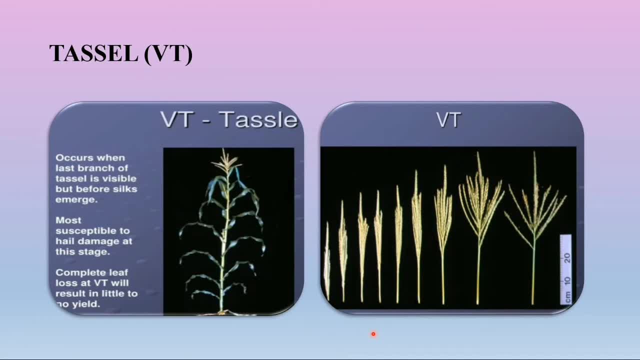 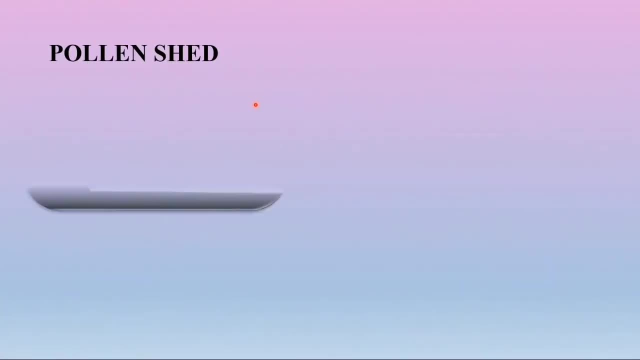 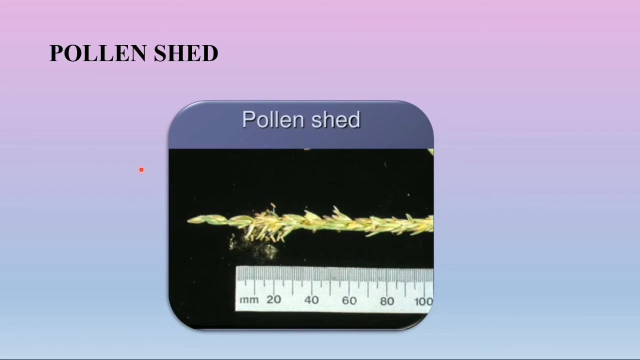 days prior to the tasseling can cause ear development to slow, resulting in lag between pollen shed and silking. this can lead to the barren ears. you can observe the pollen shed, how the pollens are shaded. the process where the pollens are shaded you can observe here clearly in this image. 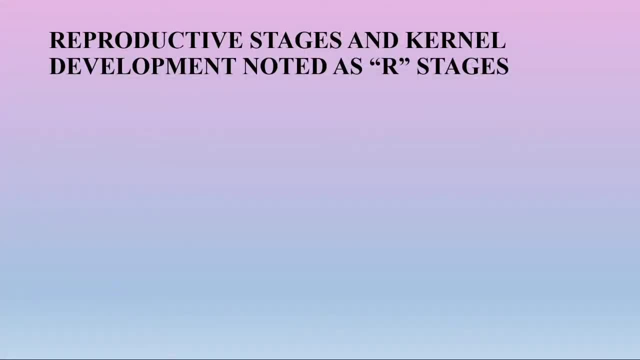 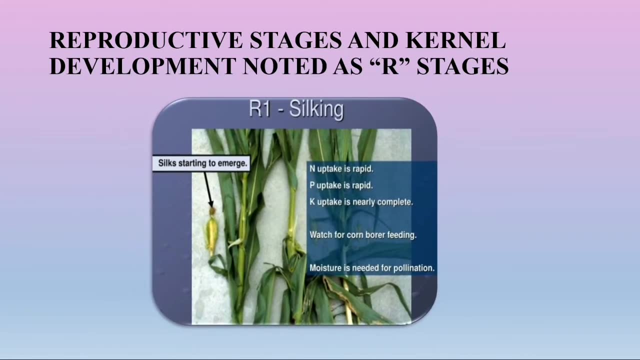 coming to the most important stages, that are, reproductive stages and kernel development, noted as r stages in the maize. reproductive stages are one like silking, where the silk starts to emerge and uptake of nutrients is rapid npk, that is npk. watch for the corn borer feeding moisture. 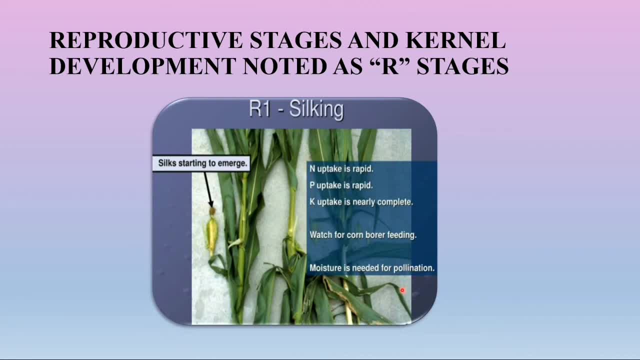 is needed for the pollination and in the silking stage. silks emerge with the growth of the corn and the growth of the maize pollen shed at the rate of 1 to 1.5 inches per day. the silks visible outside the husks. 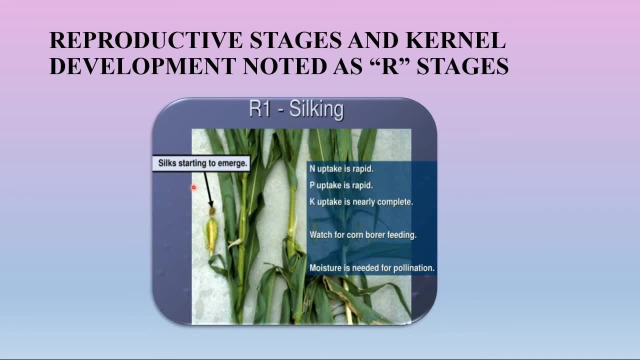 most critical stage in the development of corn plant. largest yield reduction occurs from the water and nutrients. tests at r1 takes 24 hours for the pollen grains to grow down the silk and fertilize the oval. once the fertilized, the oval becomes the kernel, generally two to three days. 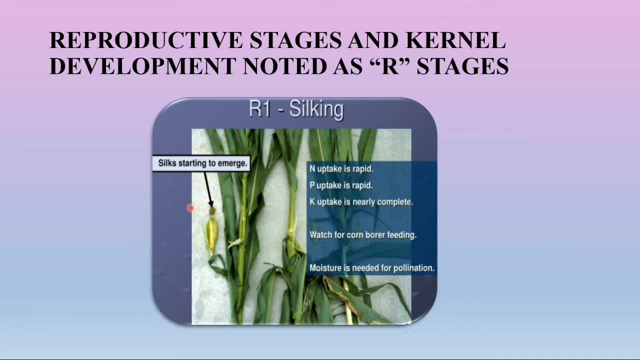 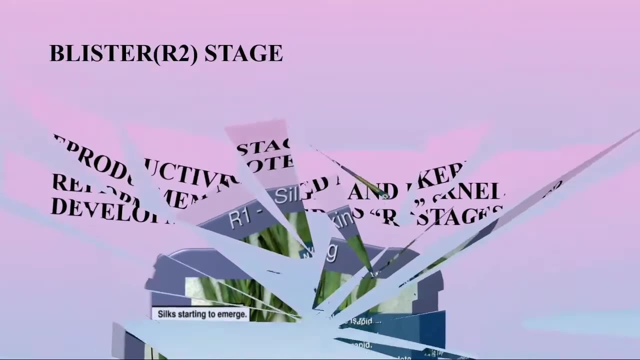 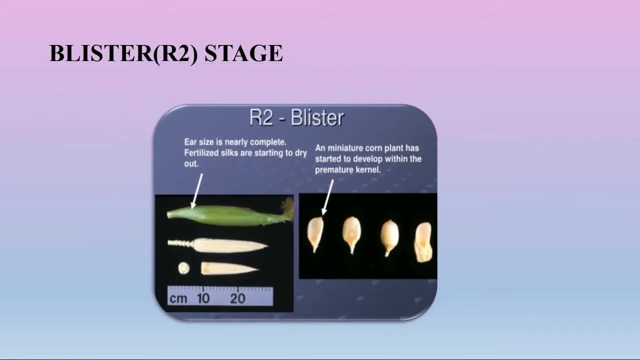 required for this silk to be fertilized on a single year. corn earworm, earworm moths may be laying eggs on the silk, so you should observe for that eggs and destroy it. and coming to the coming to the blister stage, which is r2, where you can observe the ear size is nearly complete. 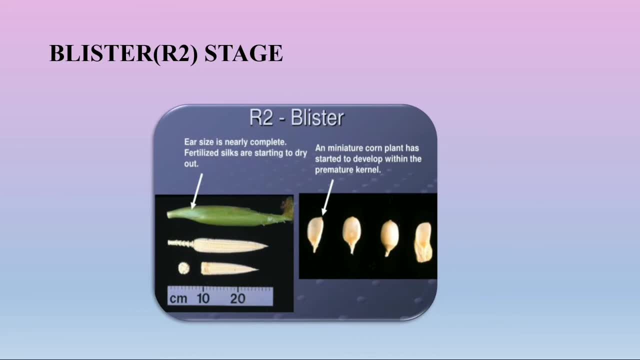 and the fertilized silks are starting to dry out. the blister stage occurs 10 to 14 days after the silking the kernels. kernels are small and watery. the silks are browning and dry. the silks will be darker under the heat and water stress, irrigation and or good soil moisture. 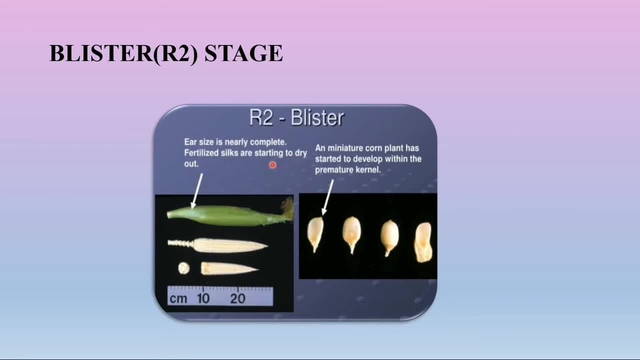 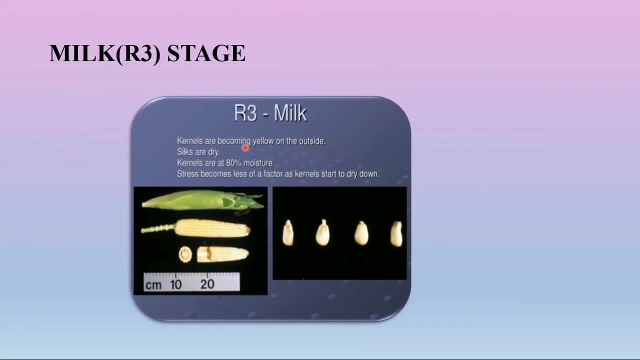 still critical for grain fill. the starch begins to accumulate in the kernel. continue to check for bank grass mite in this stage. coming to the next stage, nouth- We have the milk stage, that is R3 stage. In R3 stage it occurs at 18 to 22 days after the silking. The kernel is yellow color on the outside with a milky fluid. Here you can observe the milky fluid. grain in the corn and kernel growth is now due to cell expansion and the starch accumulation. 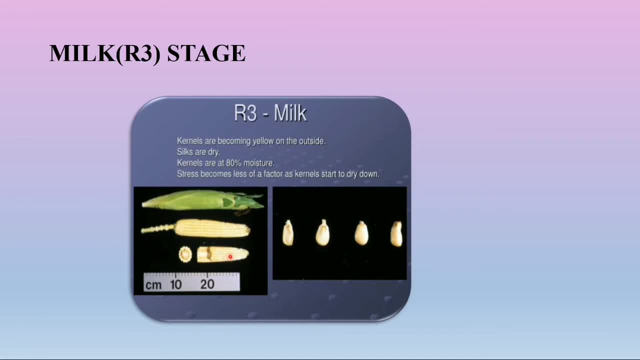 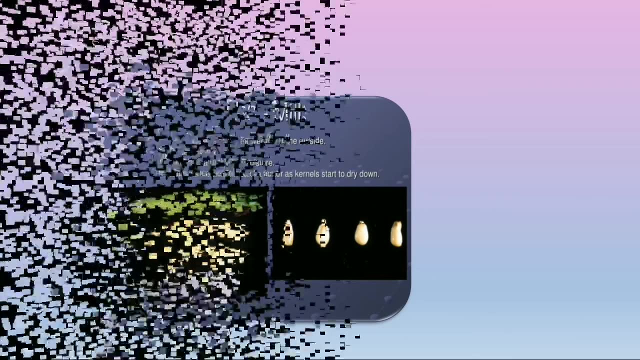 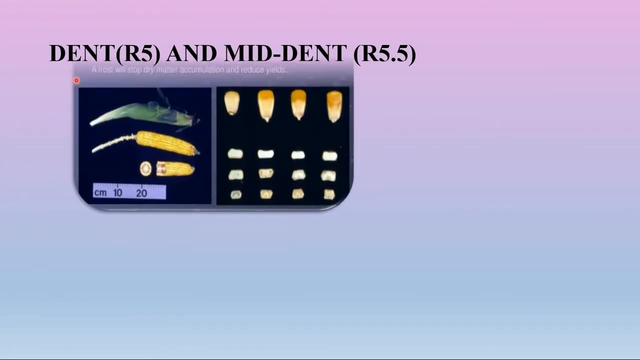 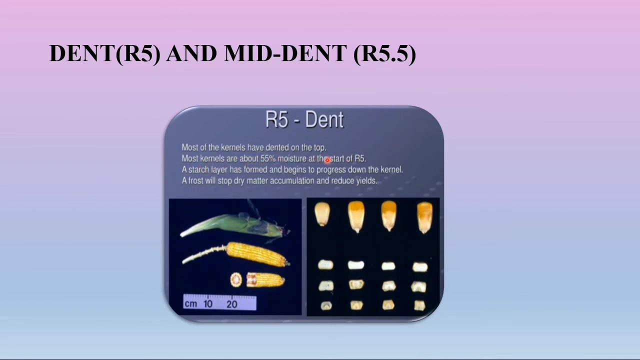 Corn, borer and mites may reach the economic thresholds. Coming to the next stage, that is, Dow stage, We have the. Now let us see about dense stage and mid dense stage. where dense stage is the most, kernels have dented on the top, and dense stage generally occurs 35 to 42 days after silking. 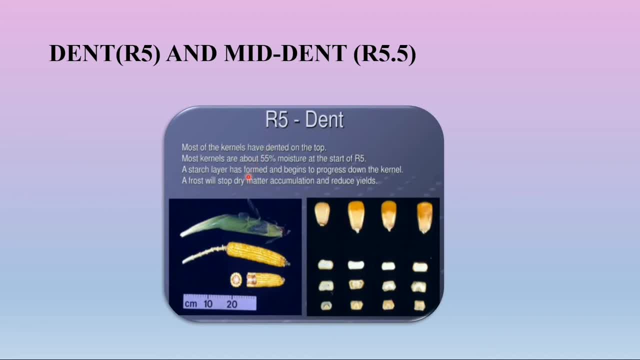 Cob is dark color, Dark red color on the majority of hybrids Coming to the mid dense stage, which is R5.5.. The mid dense stage often referred to as half milk line. As the kernels are drying down, a white layer of starch will begin to form, beginning at the top of the kernel and progress to the cob. When this hard layer reaches halfway down the kernel, it is considered to be at the half milk line stage. 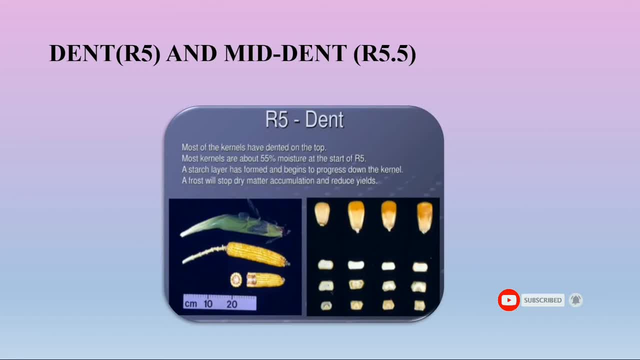 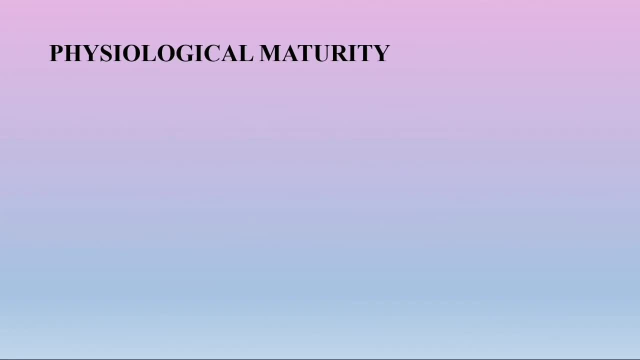 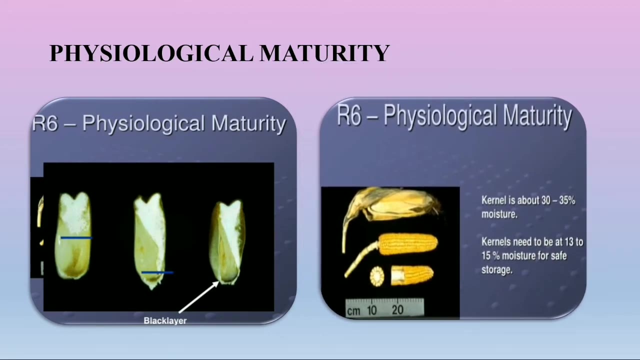 Coming to the Next stage Now, the last stage, that is, physiological maturity stage. You can observe the physiological maturity, also referred to as black layer stage, and the black layer occurs when the starch line has progressed to the base of the kernel, and this can be identified by slicing the kernel and observing the black layer stage.